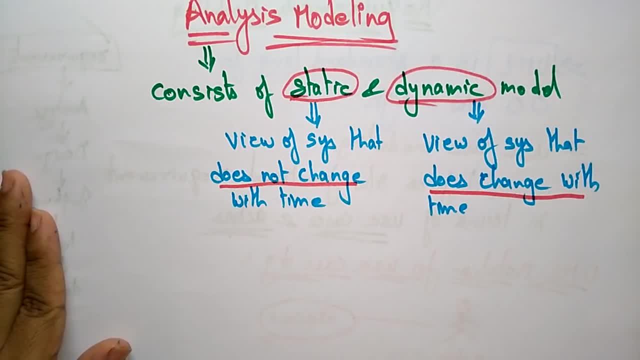 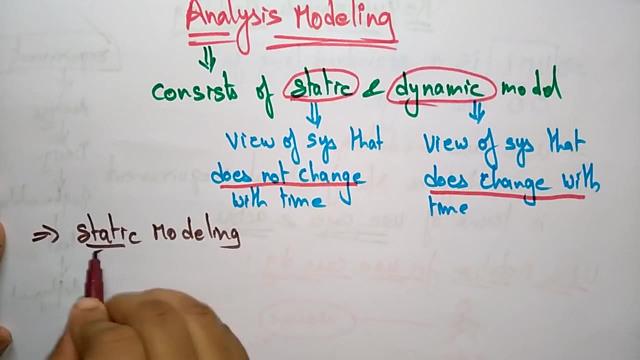 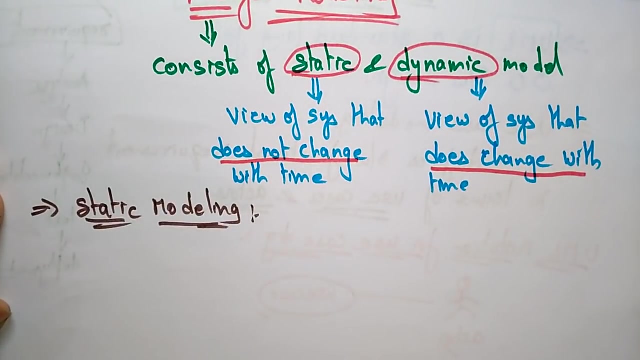 Model. Okay, So now let us see how we are representing, what are the terms that we used in the static model and what are the designs. Now let us see the static modeling. So in the analysis, modeling will consist of two models: static and dynamic. So now let us see the static model. A static modeling is defines the structural 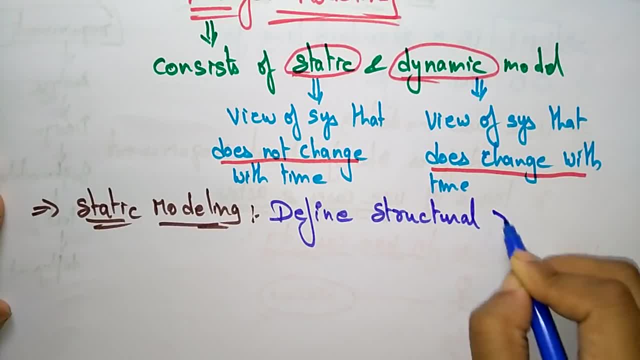 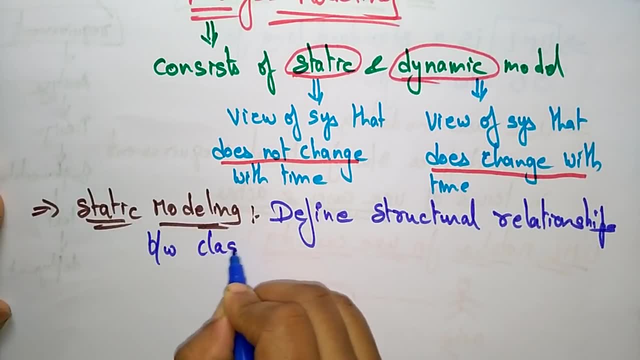 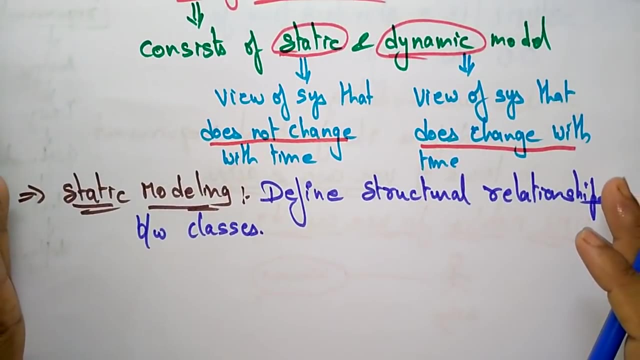 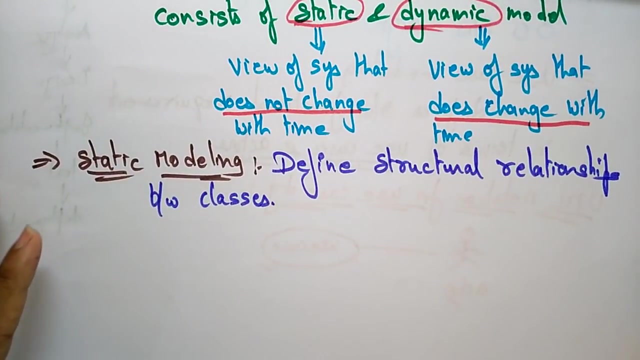 Structural relationships between classes. So static means only defines the relationship between that two: structural relationship between the classes. So here it depicts classes and their relationships on class diagrams. So, with the help of class diagrams, Let me just show you a simple example. So let us say this is a class A. 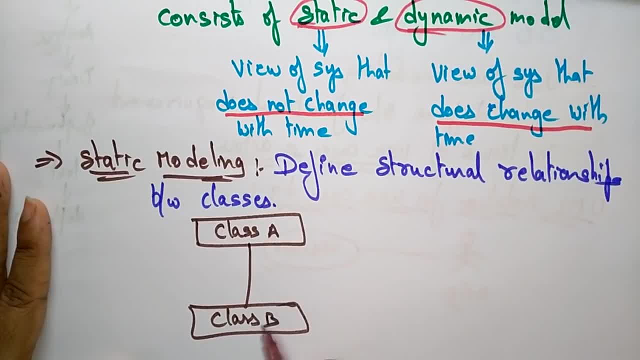 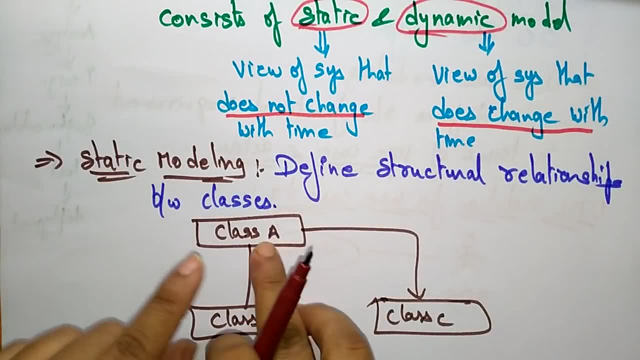 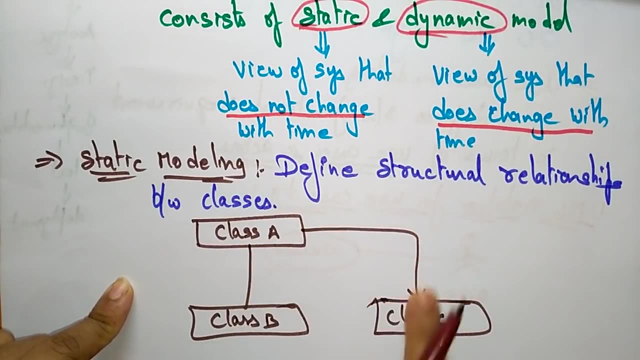 And the class B And class C. So this class is, it defines this structural relationship between classes. So this is a classes and static modeling described the structural relationship. So these are the relationships between the classes. So these relationships may be one too many. 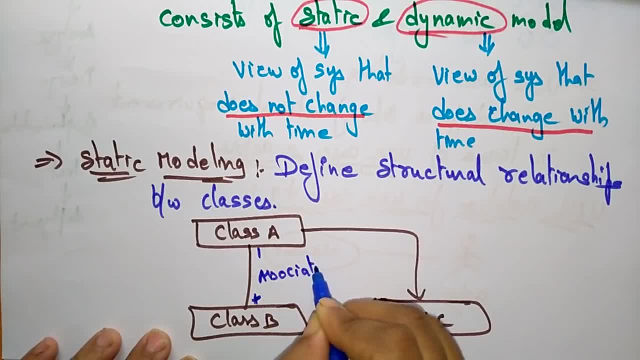 Association. So this is association relationship. So whenever a Single, Single, Single line will be there with arrows, So this indicates the association. If a solid line is there, then it is an association symbol And it is 0 to 1 association. 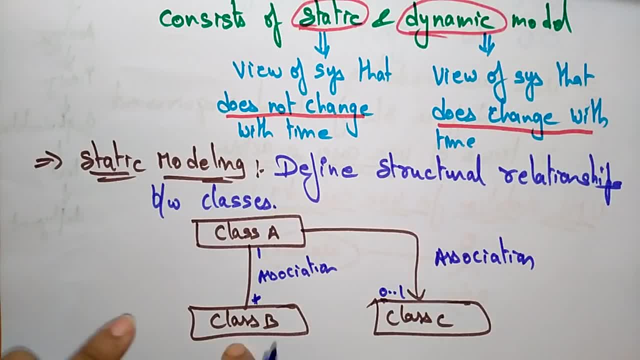 So it's just a class diagram here in the. here the class B, where the association which with the direction, in association association name is read, And whereas here the association with the direction of navigatable. So it is a navigatable, So that is the only difference. But this complete structure, you call it as it is- Can you just tell me that it shows the whole structure? 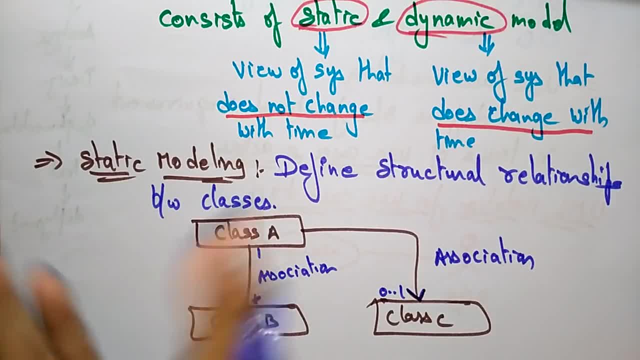 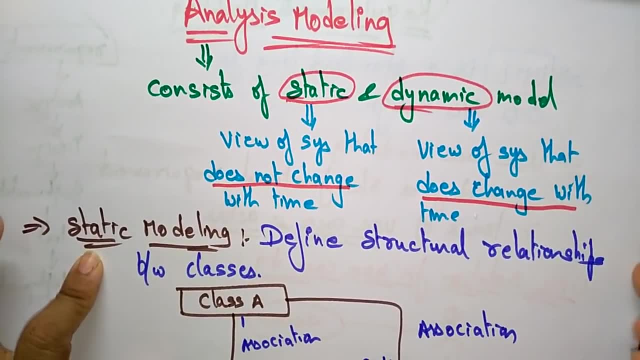 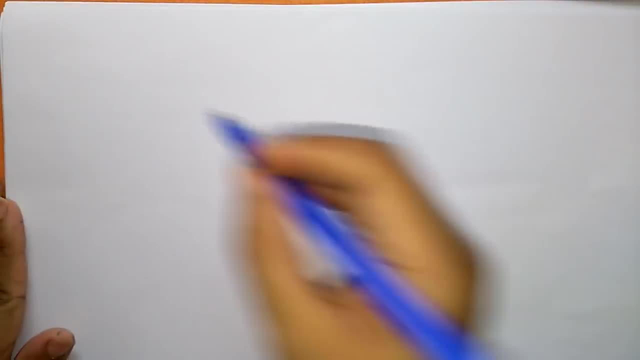 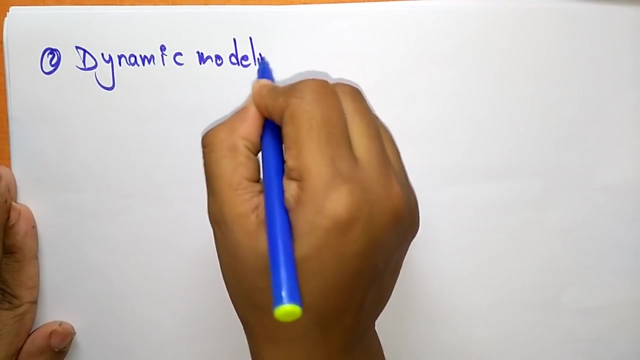 And this here it is not navigatable Again. this right here is an association, More than two here, which remains stacking Dynamic modeling, So I sell it. static modeling ease. other Defines a structural relationship between the classes 2, five, budget. And what about the dynamic modeling? 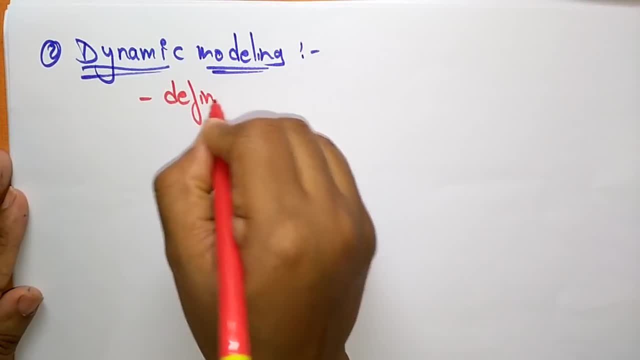 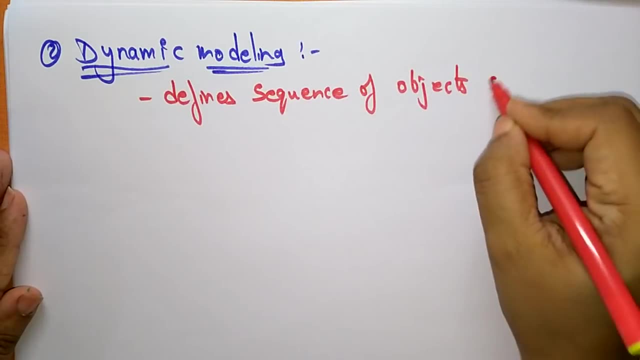 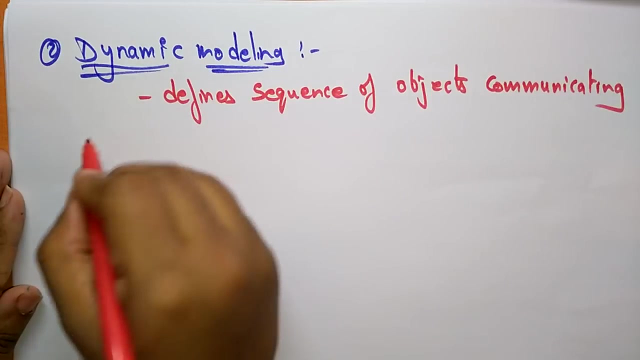 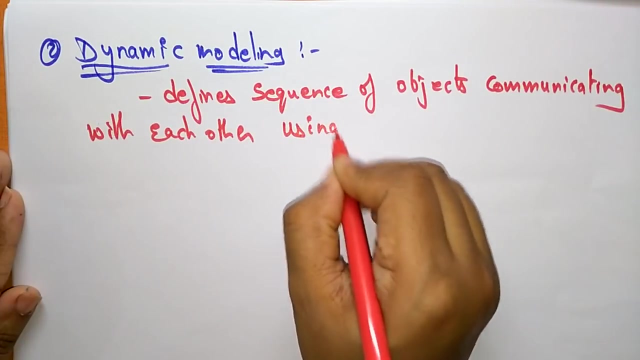 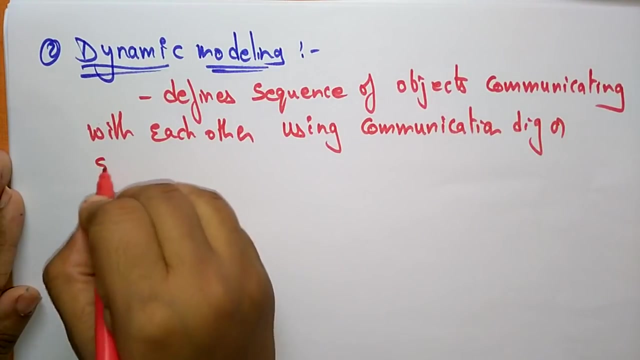 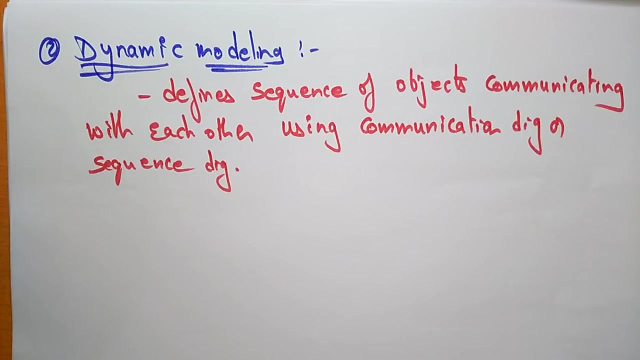 Dynamic modeling defines sequence of objects, communication, communicating, so that sequence of objects are going to communicate with each other, with each other, using communication diagram or sequence diagram. So the example for this dynamic modeling: we use the sequence diagram. So, whereas in static modeling we use the class diagrams and in the dynamic modeling we will use the sequence diagrams. 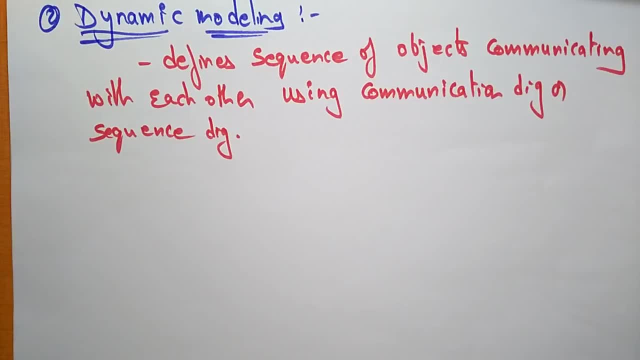 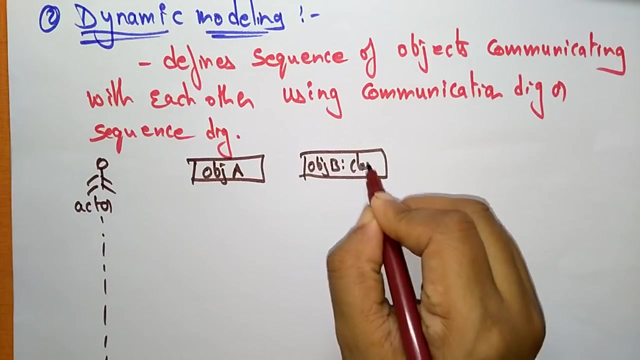 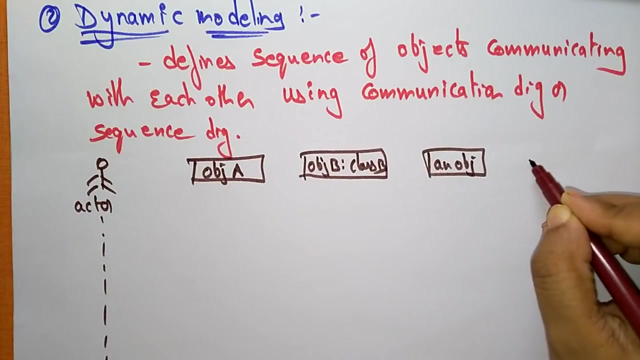 So now let us see the UML notation for the sequence diagram. Here is an actor, object A. So here the sequence of actions will be communicating between the objects: Object B of class B, any other object which is related to another class. 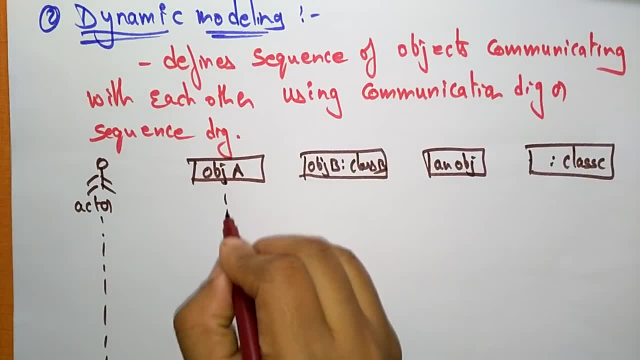 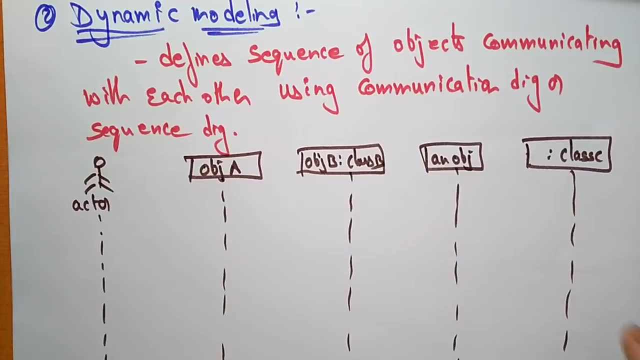 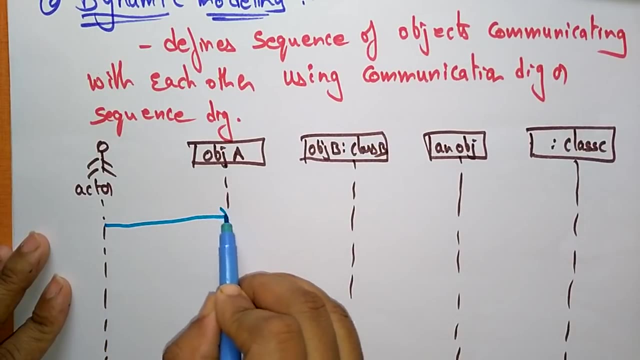 And class And class And class C. So dynamic modeling means it changes with the time. So this sequence diagram indicates the time sequence. So at a particular time the message will be: First: the actor is communicating with the object A, that is, input message. 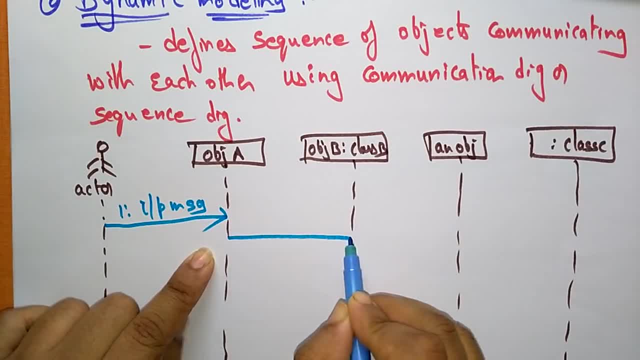 After a particular time, the object A is communicating with object B, which is represented in class B. So two: internal message is passing Internal message, And three: another message is sending from one object to another object, Just interacting a communication. that too in the form of sequence diagram. 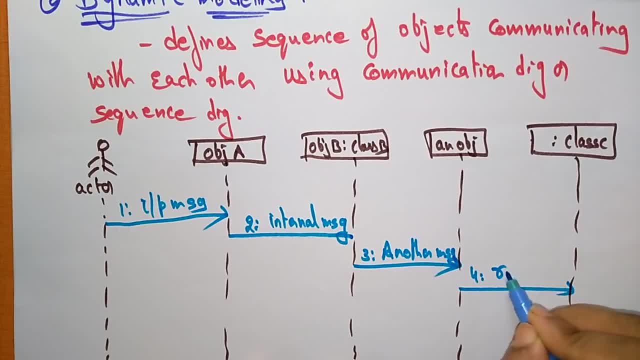 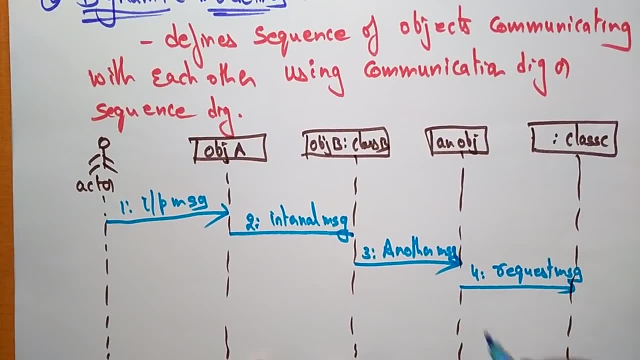 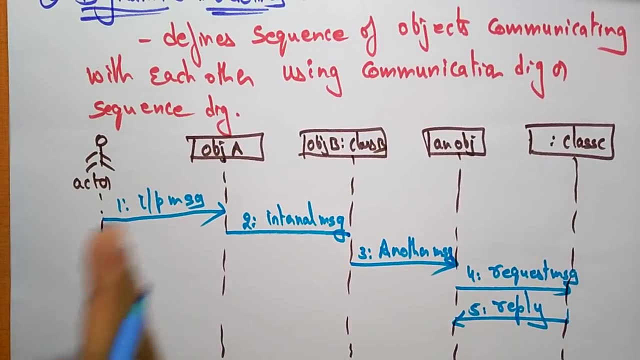 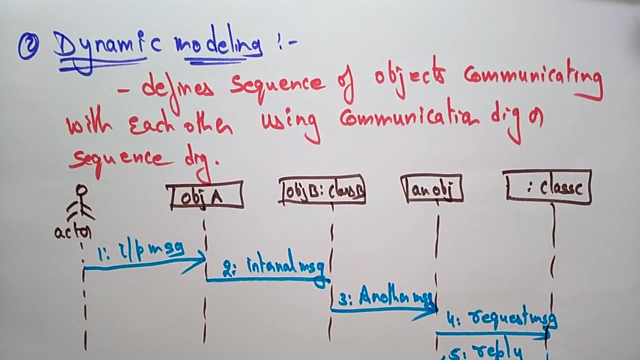 And here the fourth sequence is it requests for message. So after sending one message, this an object is requesting the class to send another message. so this class is going to reply in this sequence. so this is a sequence: first step, second step, third step, fourth and the fifth. so this is dynamic modeling, so the analysis modeling. 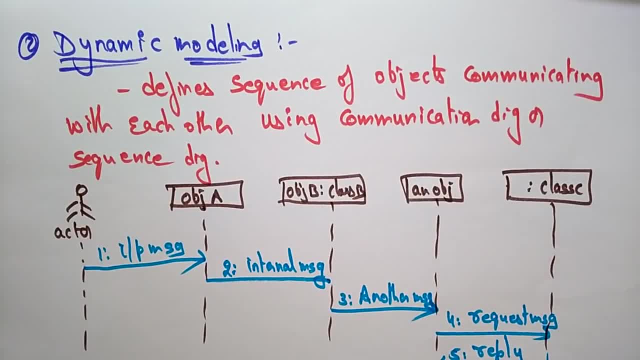 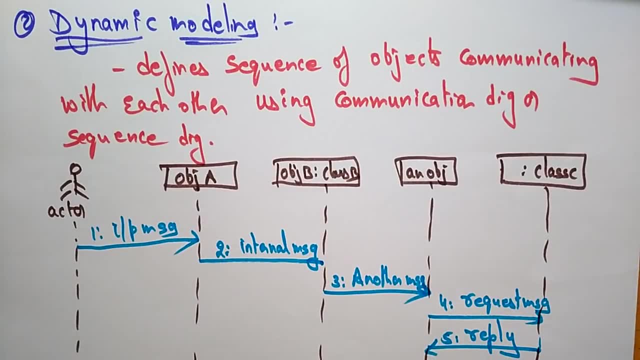 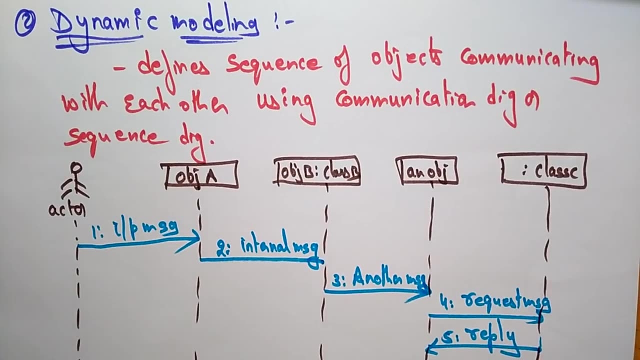 can be divided into two types: static and dynamic. static only defines the structural relationship between the classes, whereas the dynamic modeling is just defines the sequence of objects, the sequence of objects communicating with each other using sequence diagram. thank you.